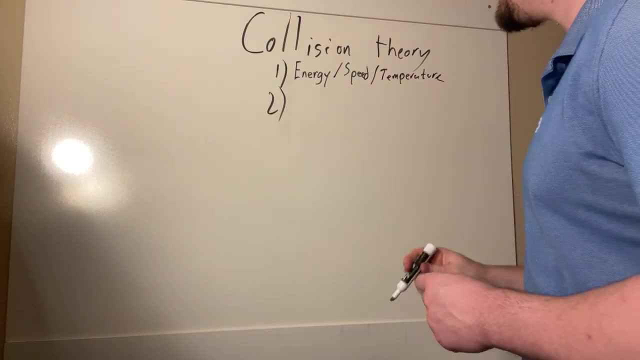 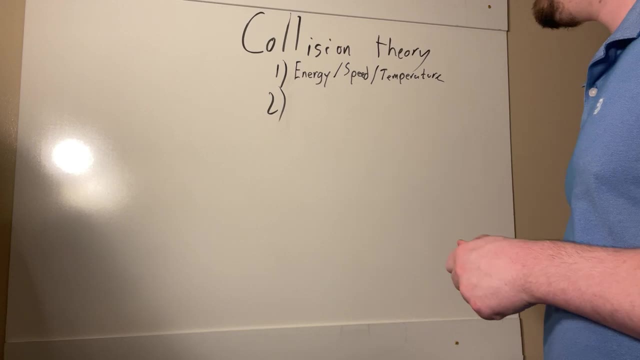 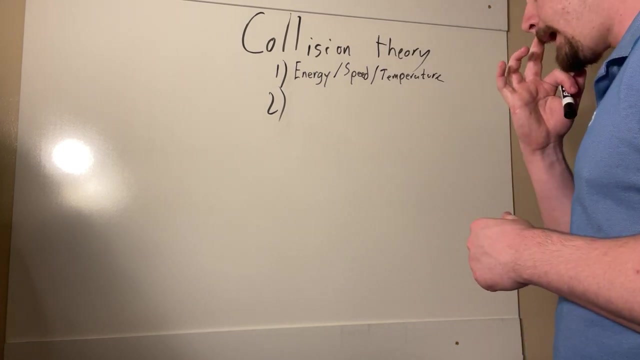 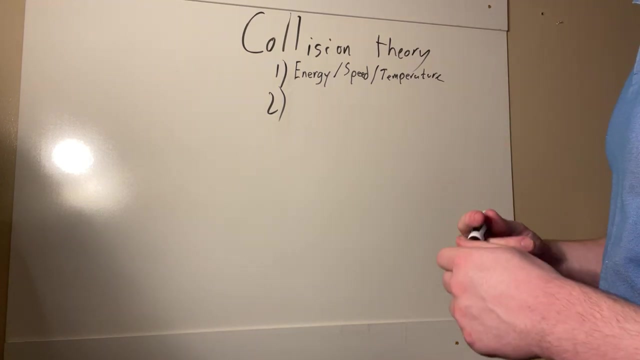 So the reason why there's so many slashes here. So when we think about atoms and molecules having a lot of energy, what that really means is that they're moving. They're moving at higher speeds, And how we detect that, How we detect that at a large scale, is the temperature of said 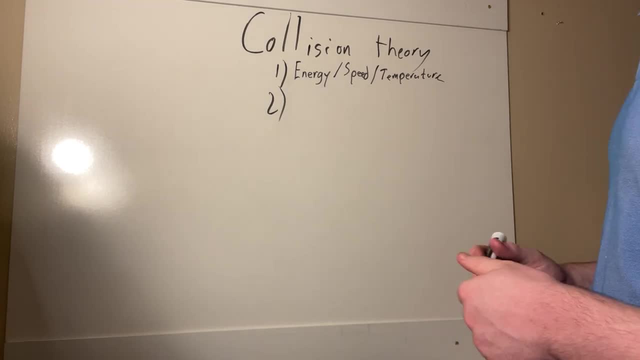 Of whatever we're talking about. So you can think of it like this Hot water is moving at a faster speed. The molecules in The water molecules are moving at a faster speed than cold, Colder water. And you can think of it like: 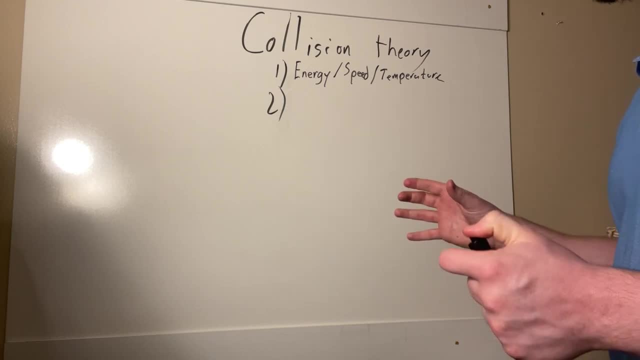 Ice is so cold that the water stops moving, which isn't entirely true, but it's a good way to think about it. If something has more energy, it's going to be moving faster and it's going to have a higher temperature. 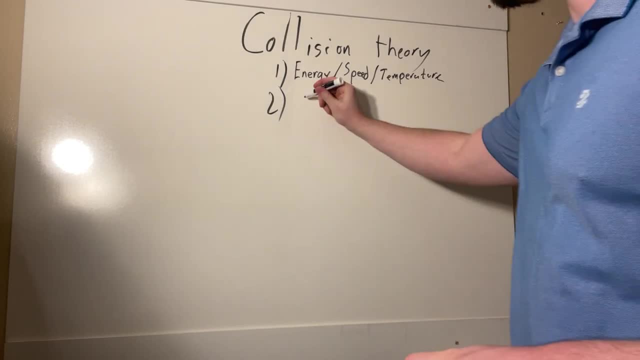 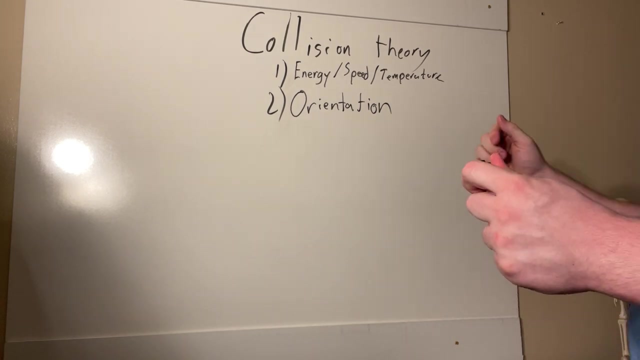 And then number two is going to be orientation: Orientation, So they have to hit in the right way. This is going to be really important in In organic chemistry, Because if, If something doesn't react, If something doesn't, If two molecules don't hit in the right way, then they're not going to react. 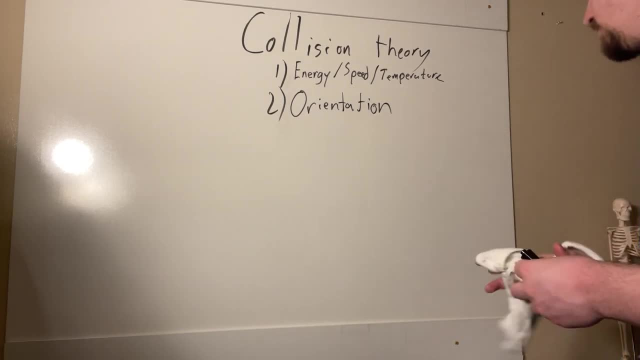 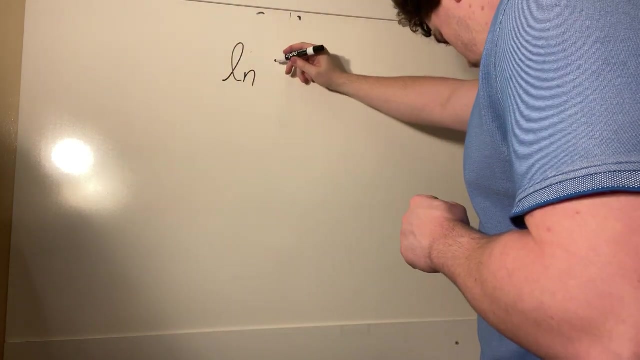 So, Now that we know these two things, Let's move on. So we are worried about the temperature and the orientation when it comes to collision theory. So now this brings us to our equation, The main equation for this part of the, This part of kinetics. 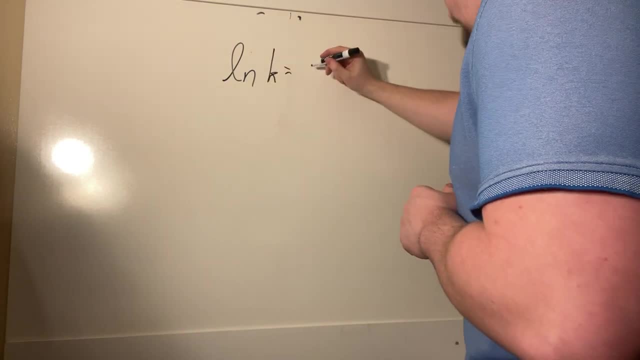 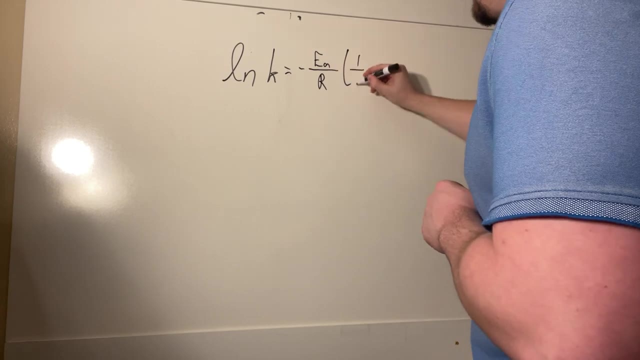 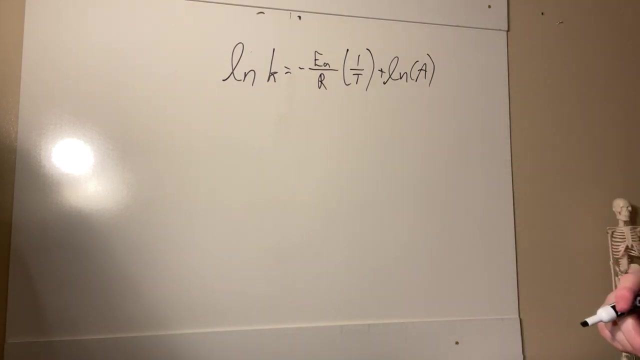 So LNK equals NER 1 over T plus LNA. So this is going to be our main reaction. So you can actually see what You can actually see the collision theory in this equation. So the first thing with collision theory is that it has to be. 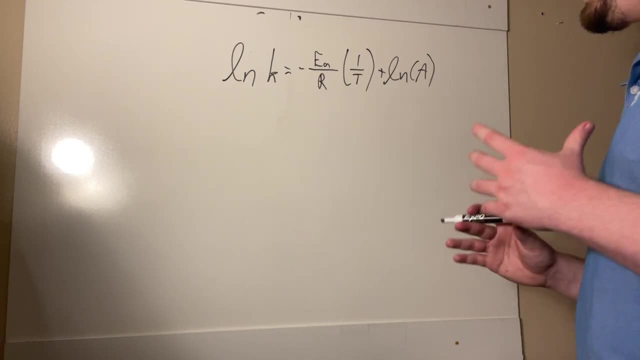 It has to have enough energy, It has to be moving fast enough, It has to be a certain temperature. Which temperature is part of this equation? So There's part of our collision theory shining through The other part. Orientation Shines through in this LNA bit. 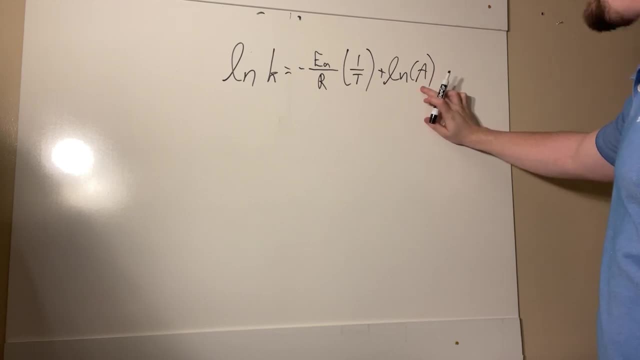 So what A is? This is called our orientation factor, Which is important because If we don't have this, If we don't have this, We're missing out part of our equation That we'll need to figure out any of these other values. 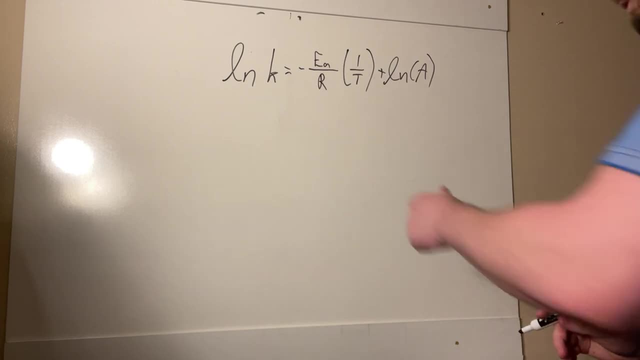 That we'll need to figure out any of these other values. So let's look at it. And R- R is just a constant And it is equal to 8.314.. 8.314.. And I'd have to look up the. 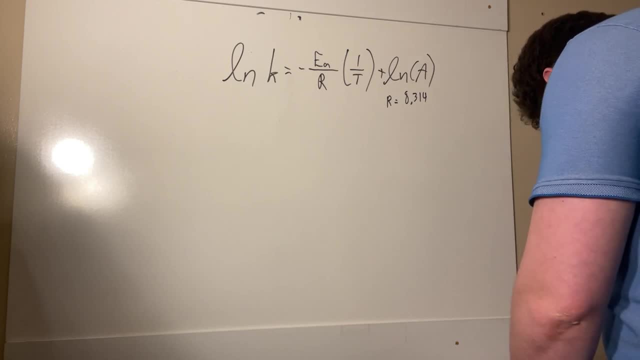 And I'd have to look up the Units on that. Units on that. Units on that. Yeah, I'll have to look up the units on that, But It's a different R value than you used in the. It's a different R value than you used in the. 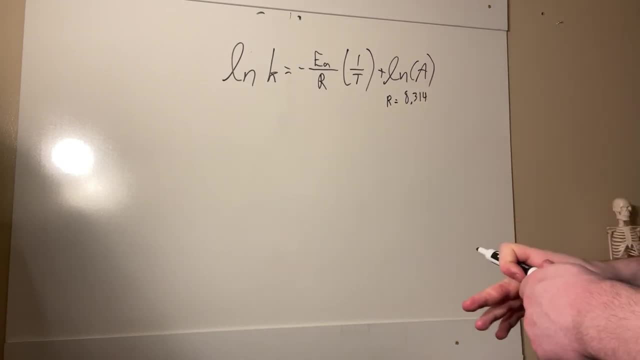 In the gas laws section. So Now that we know what that is, Now that we know what that is, Let's talk about how this is going to be asked. Let's talk about how this is going to be asked In your practice. problems and such. 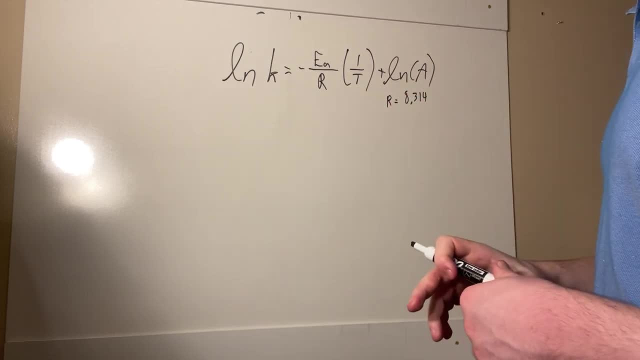 So notice that we have 1,, 2,, 3, 4.. So notice that we have 1,, 2,, 3, 4. Different variables. So, just like in the past, they're going to be giving you. 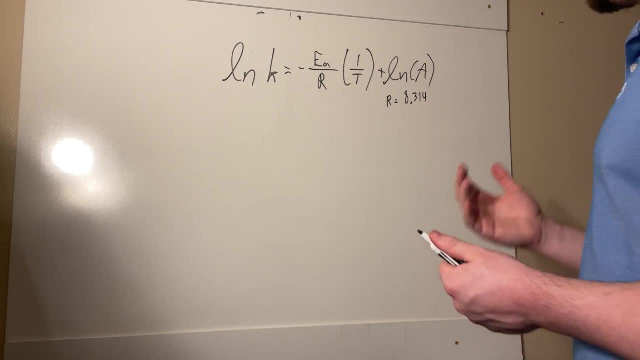 So, just like in the past, they're going to be giving you Three of these variables And you're going to be finding the fourth one. Most of the time, they're going to be asking you For two of these, And then you're going to have to find the rate constant. 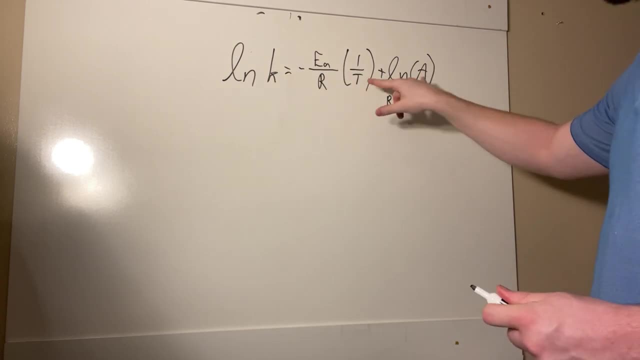 You're going to have to find the rate constant Or the activation energy, because these two Are the biggies. These two are more side. These two are more side. They're more push to the side, But most of the time you'll be asking for these. 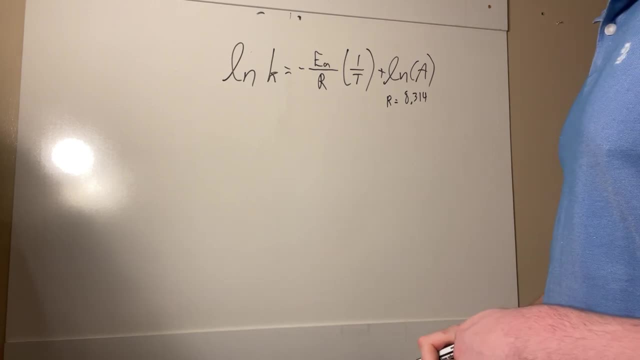 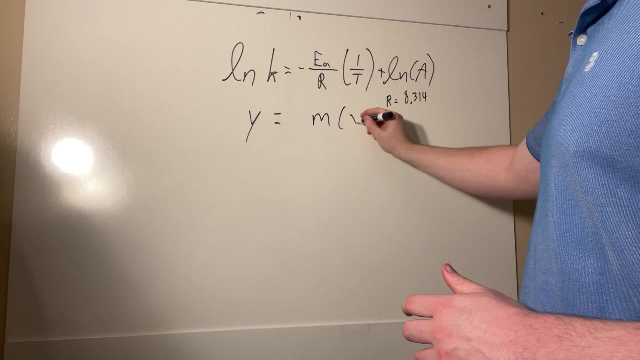 But most of the time you'll be asking for these. But if you can find these, you can find the other ones. So let's talk about the Those astute among you. Those astute among you. a little reminder: the slope of the line is y equals mx plus b. Now, in this case, 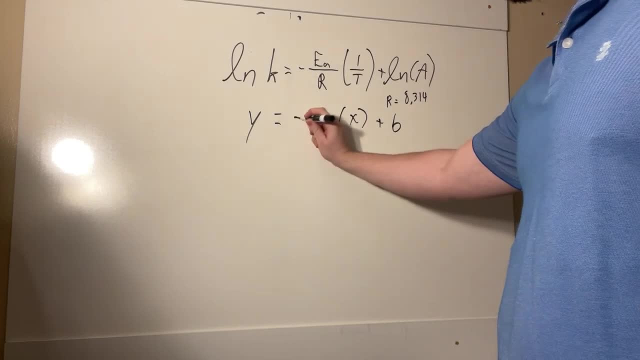 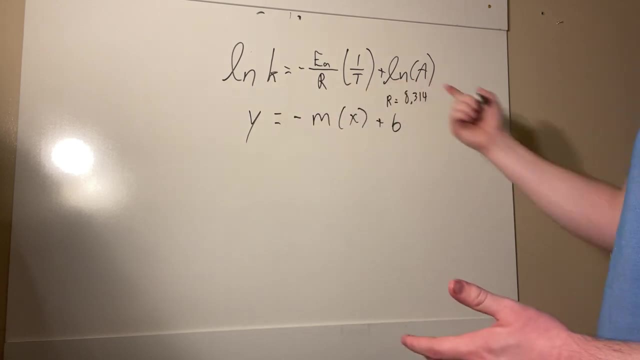 let's, let's just talk about a negative, a negative slope. So you'll look at this and you'll say, hey, the, the Arrhenius equation looks just like this line of a slope. You know l and k is your y value. this: ea over r is your slope, 1 over t is. 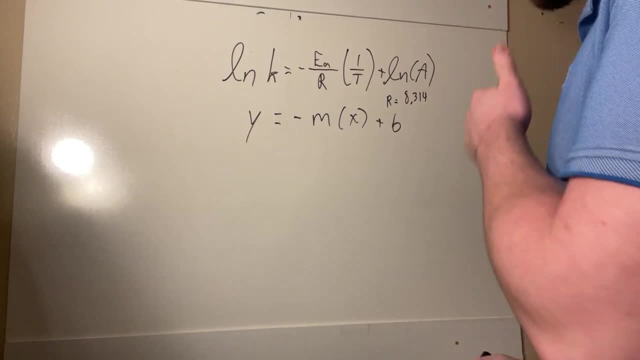 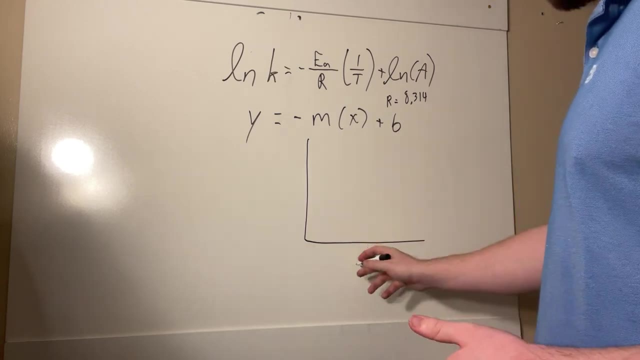 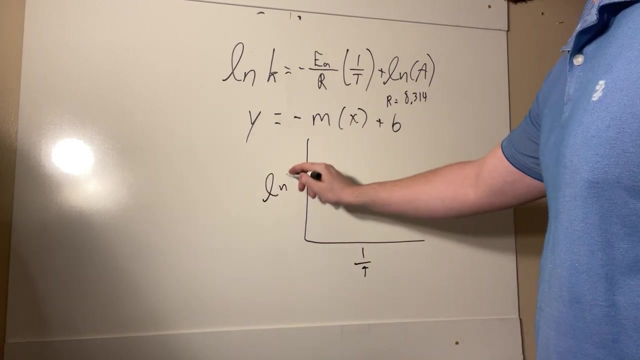 x and then b is your the natural log of the orientation factor. So what? what if we were to make a graph of this? So x and y? so x would be 1 over temperature and then y would just be l and k, and we know that the line is going to go be going. 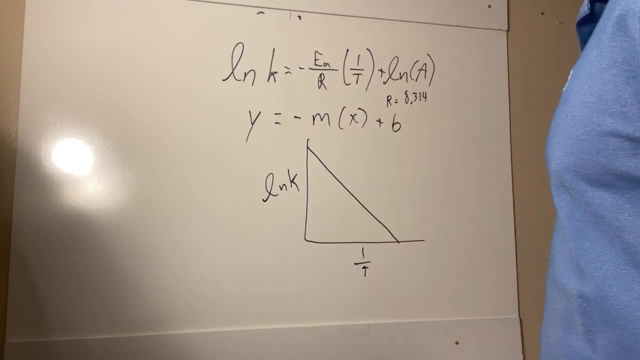 down because that's what we got up here. So if we were, if you, if you were to have a lab about this, or if you were given values of tip temperature and then the rate constant, then what you could do is you could plot the inverse of temperature. 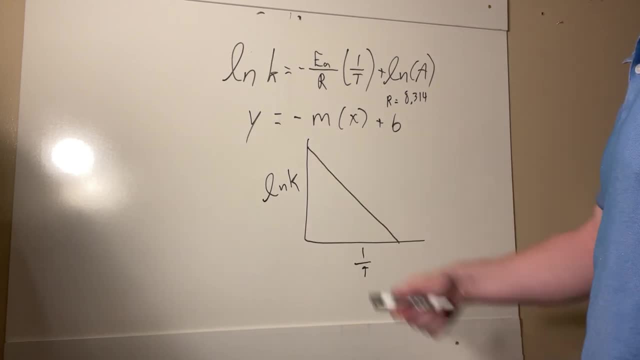 and the natural log of k, and you would get a reaction like this. Now, let's say, you don't know the activation of energy or the orientation factor. Well, you could find those by generating a line of best fit- this in this case- and you 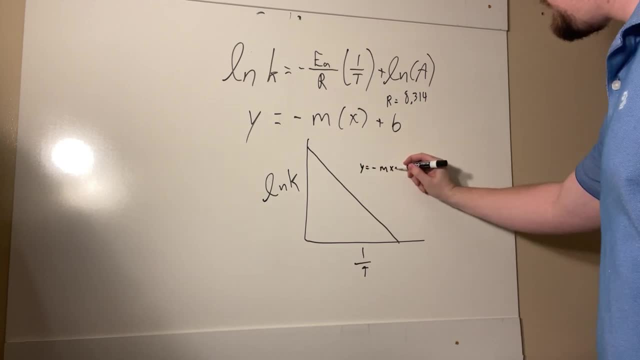 would get this equation And you could find m. you could find the activation energy because m is equal to the activation energy over r. So all you have to do- and r is a constant, so you would just have to times it on both sides and you would get the activation energy. 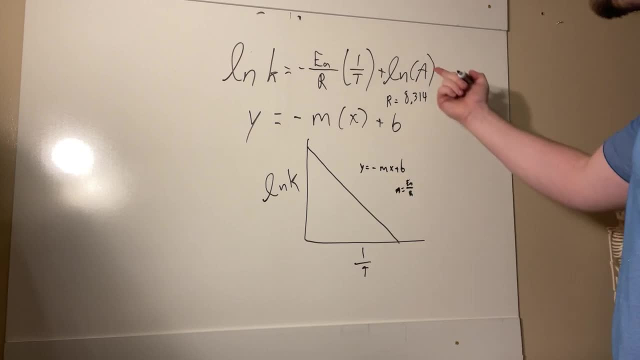 That's super useful. And then, if you wanted to find the orientation factor, you would just have to, you would. you would just have to undo the natural log. that's there. So b is equal to the natural log of a. and then you would just have to, you would just have to e, You'd have to e both sides. 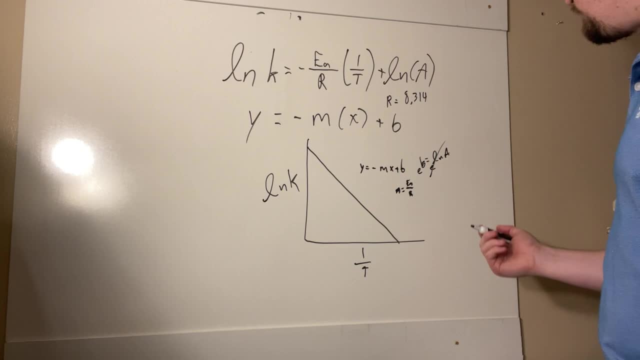 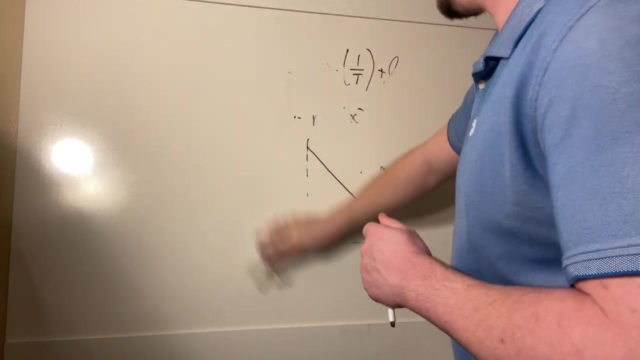 so e and natural log would cancel, and then e of b is equal to a Super useful stuff here. So for you to just for you to just just see, Now there's another thing we can do with the Arrhenius equation, And what that is. 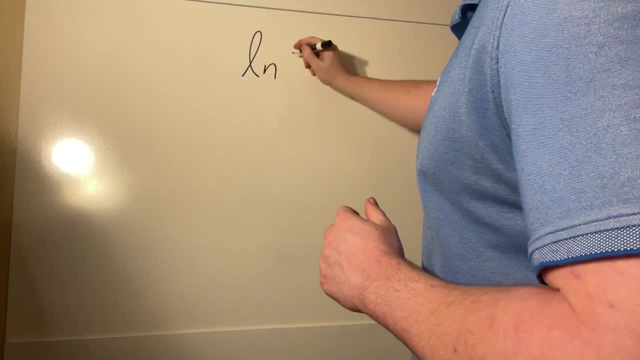 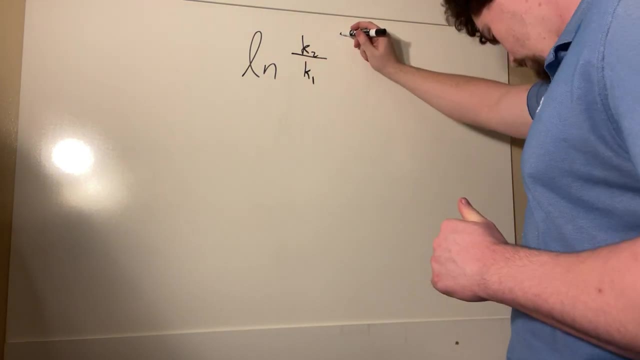 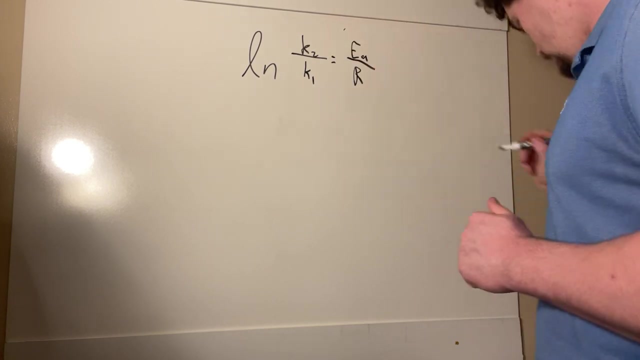 going to be. we're going to be comparing two different, two different things. So it's going to be ln rate constant two over a rate constant one, and this is going to be equal to e- the activation energy- over r. Then it's going to be r over a constant two. I'm going to take out the air and I'm going. 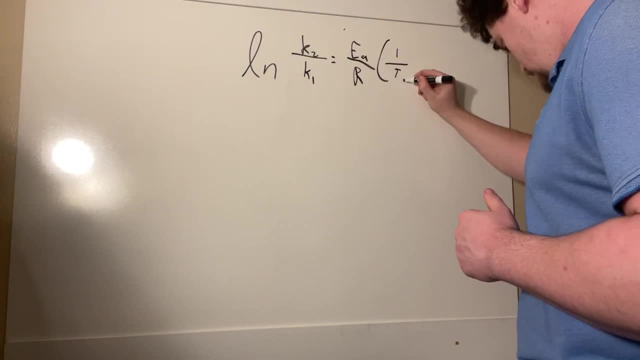 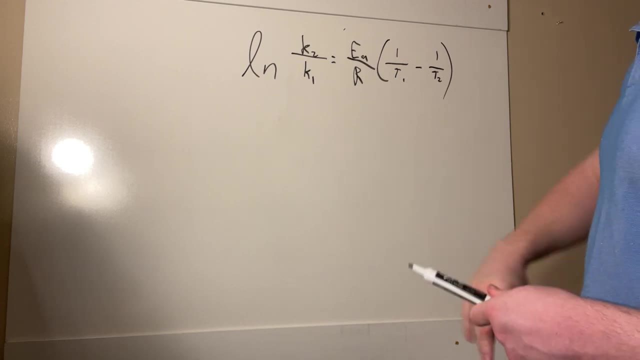 to take off the air. Gotta do that kind of thing, And since I have another equation that's almost useless, this is just my luck- Let's try it again and see what else happens. 1t1 minus 1t2.. So this is a pretty similar notice that we're given 1,, 2,, 3,, 4,, 5, 5 values. 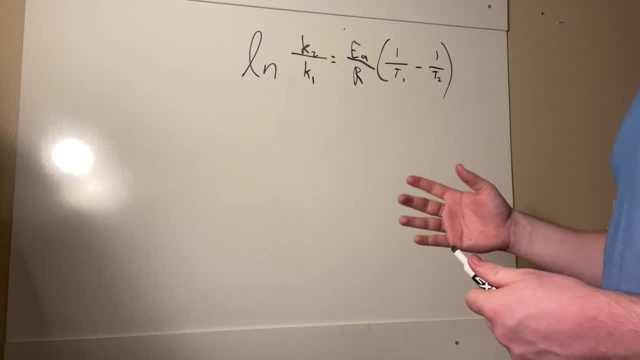 So the only way this is going to be different- so is there your teacher or practice problem- is going to give you four variables and you're going to be looking for the last one, Um, and, based on my experience, most of the time they're either going to be asking um for one of 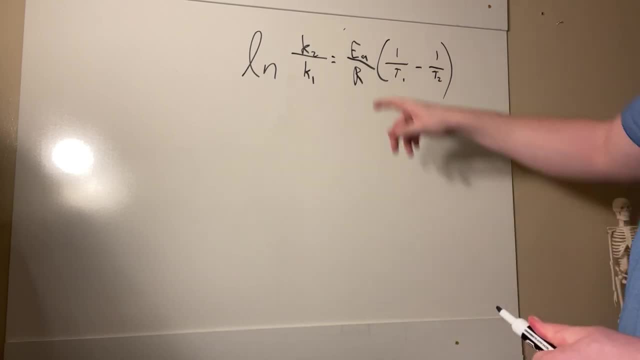 the rate constants or they're going to be asking for one of the temperatures. Sometimes I ask for the activation energy, Um. but if you can, if you can solve for any one of these, you can solve for uh the rest of them. We just have to know our basic algebra skills. 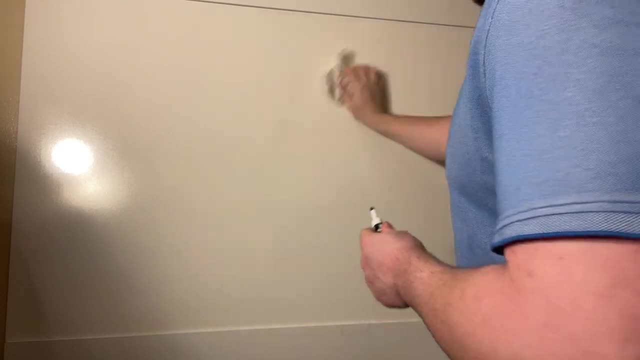 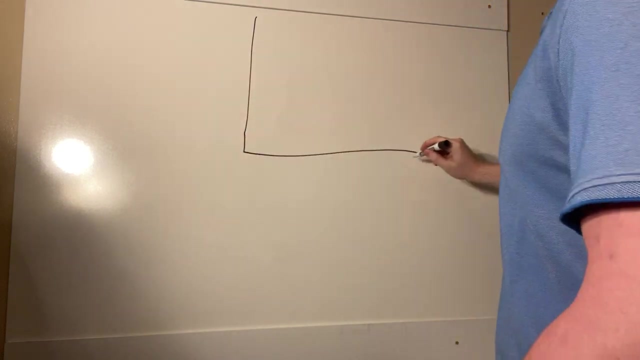 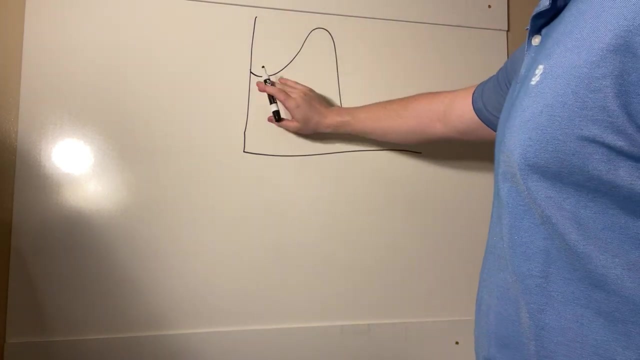 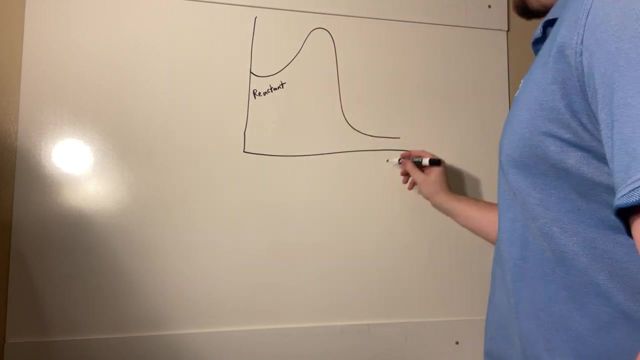 All right, Um, and then just to talk about what activation energy is: uh, let's, let's review that. So, what activation energy is? let's just write a simple reaction diagram. So the left side is going to be your reactant side, whereas the right side is going to be your product side. So left is your. 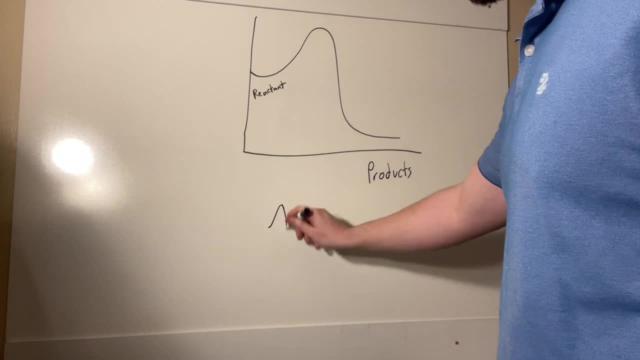 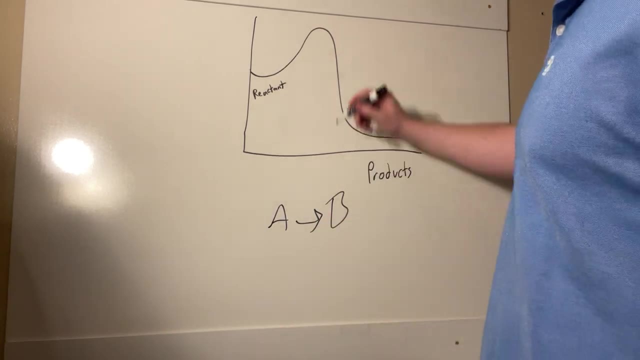 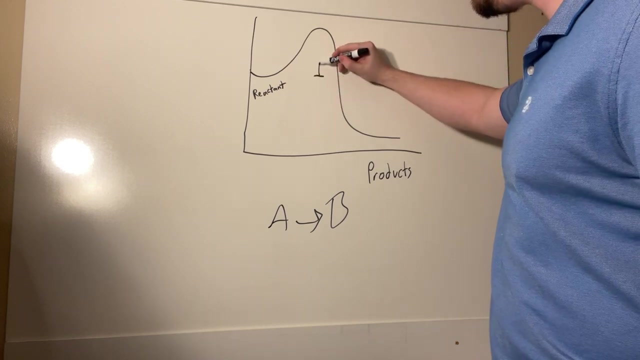 reactant right is your product. That's easy, because let's just say we're talking about A going to be. Your reactants are on the left, products are on the right- Super easy. So your activation energy is from the reactant side to the top of this little heel and this is your. 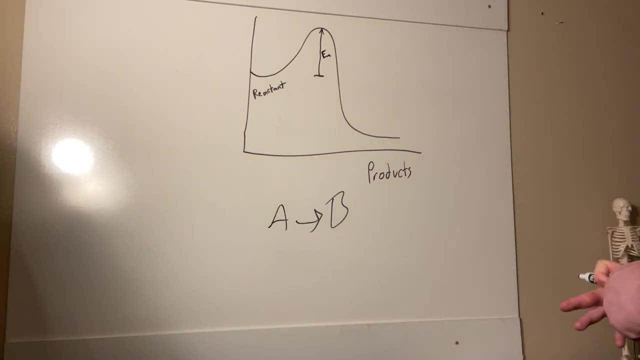 activation energy. So you're like: what's the big deal? Well, if this activation energy is super high, then it's going to be hard for your reactants to get enough energy to make it over the heel to the products, And this can be. 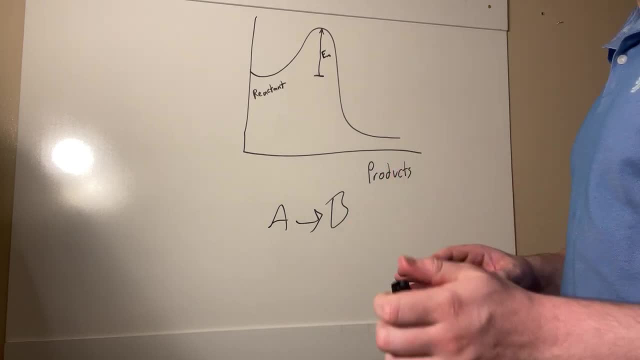 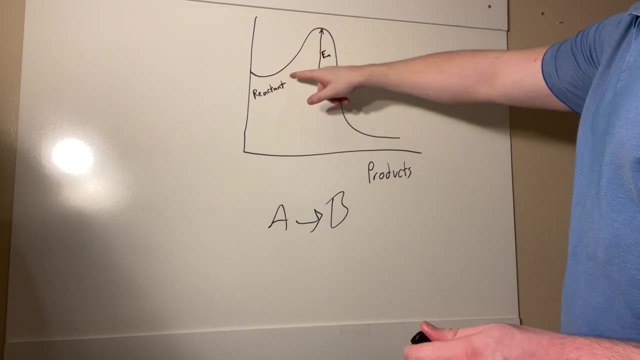 very intuitive. if you think about wheeling a wheel up here, So think about: it's a wheelbarrow, so you're trying to get it up. The steeper this heel is, the harder it is for you to push that wheelbarrow up. 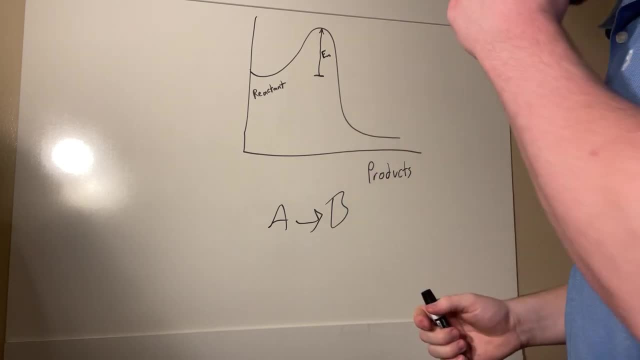 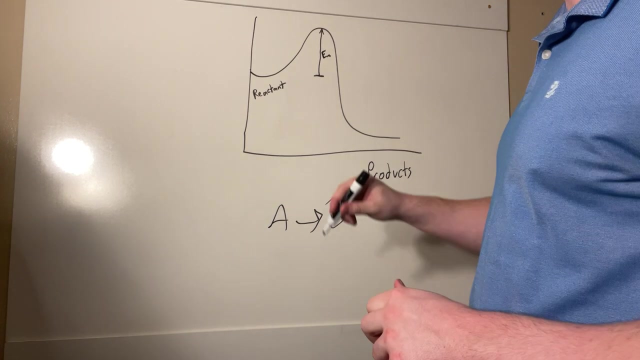 Whereas if it's smaller, it's not going to be as hard for you because the heel is not as big. So so there's that. Another important thing here that we will talk about is something called a catalyst. So what a catalyst does. 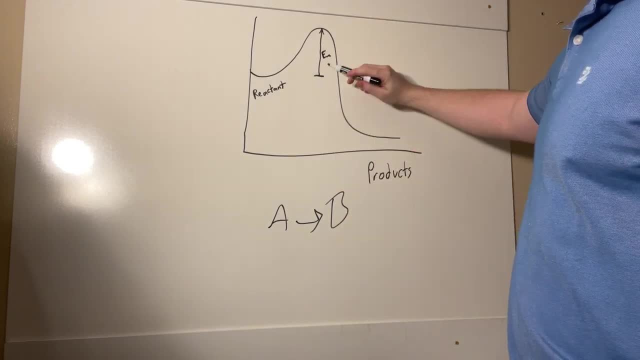 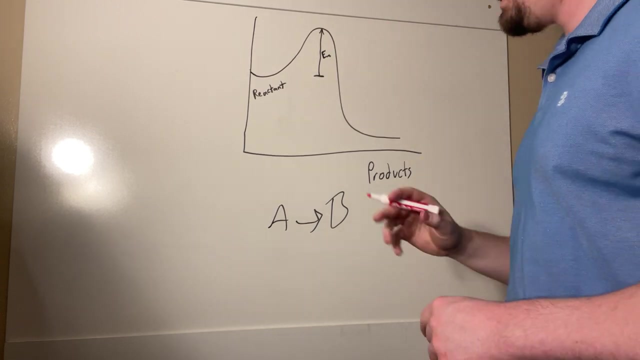 a lot of people think that catalyststheir physical move this activation energy, And that is not true. Catalysts do more than that energy and that is not true. catalysts do not do anything with the activation, with the activation energy of this. we're gonna use this red marker here to show 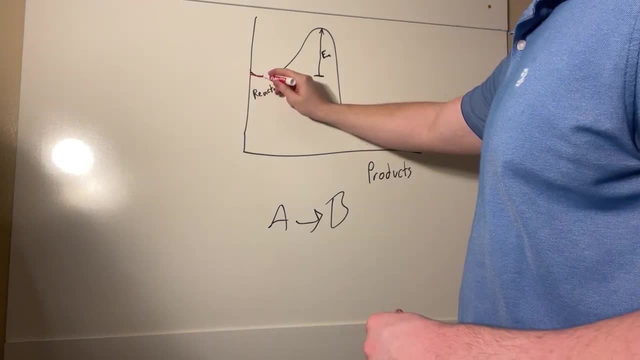 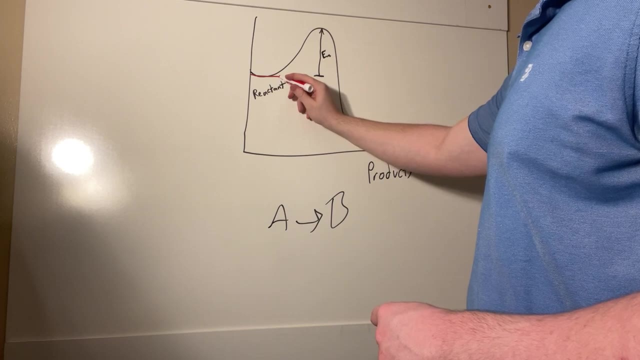 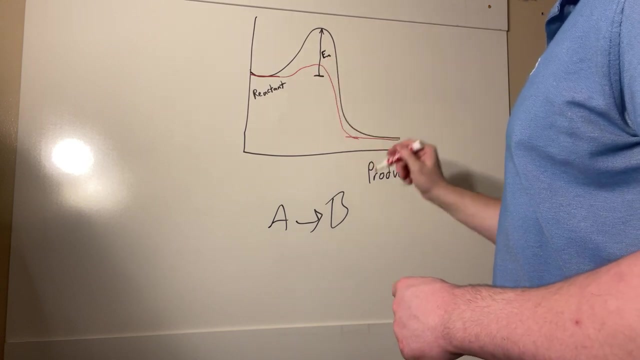 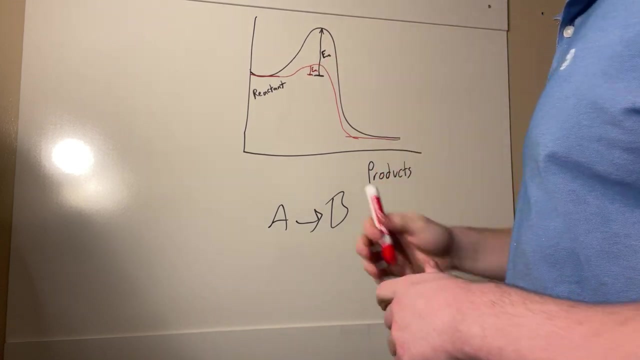 what a catalyst does. so a catalyst is going to, it's gonna happen. it's gonna have the same reactant spot and it's gonna have the same product spot. what it is going to do. a catalyst provides a different pathway to do the same reaction. so notice that in this one, the activation energy for the catalyst is a.